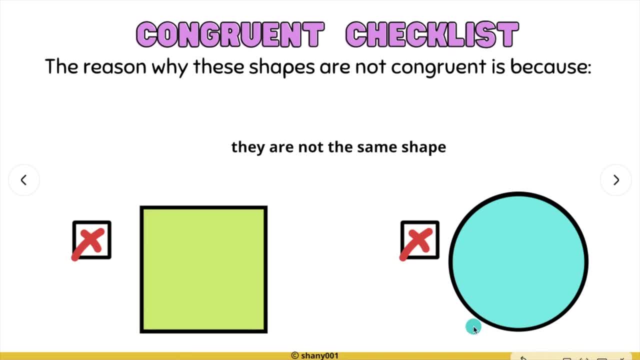 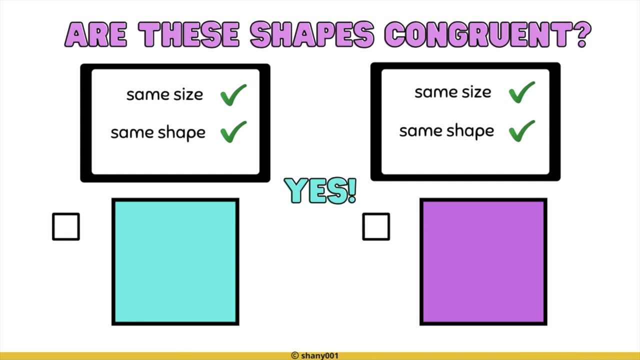 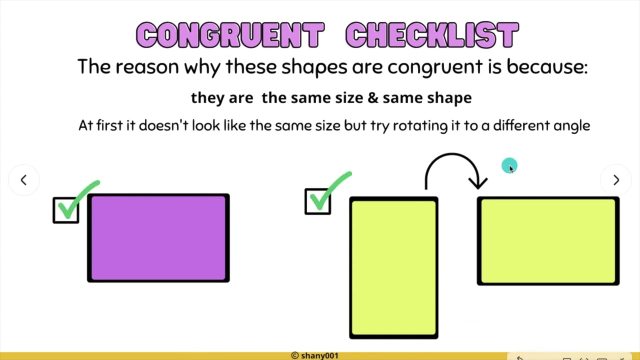 This is a square and this is a circle. Are these shapes congruent? Yes, they are. They are the same size and same shape. Are these shapes congruent? Yes, they are the same size and the same shape. At first it doesn't look like the same size, but try rotating it to a different angle. 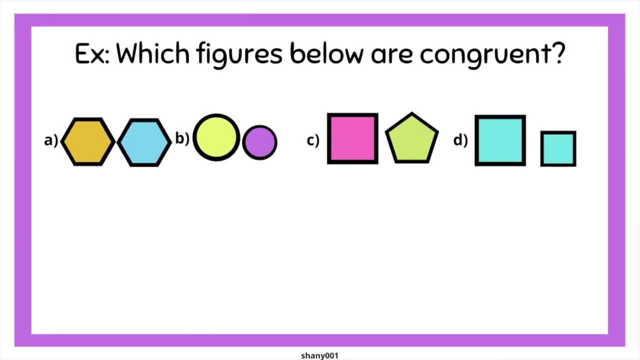 Try rotating it to a different angle. Which figures below are congruent? The answer is: A- They are the same size and the same shape. B is not correct because they are not the same size. C is not correct because they are not the same shape. 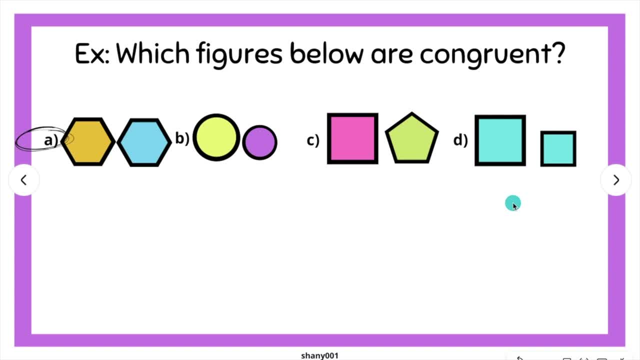 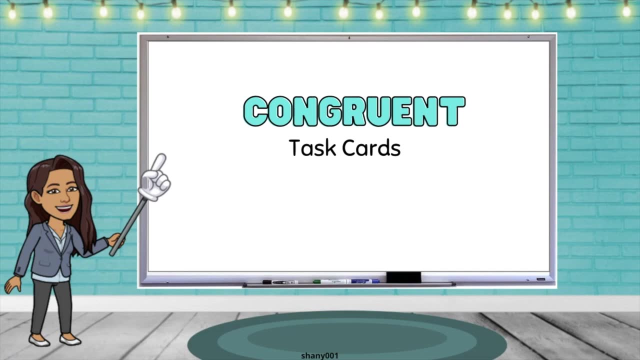 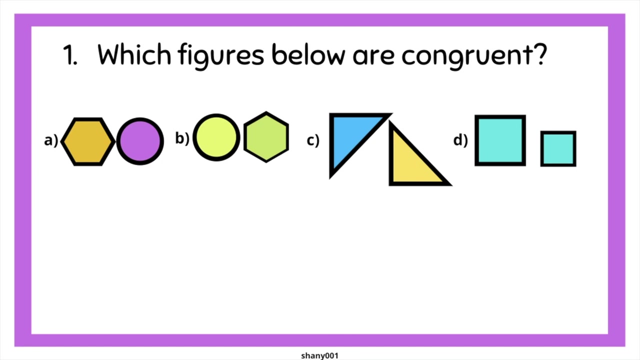 D is not correct because they are not the same size. Congruent means same size, same shape. Here are some more task cards on congruent figures. Number one: Which figures below are congruent. Number two: Which figures below are congruent. 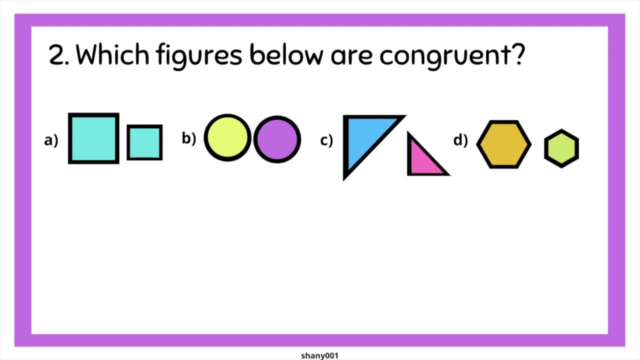 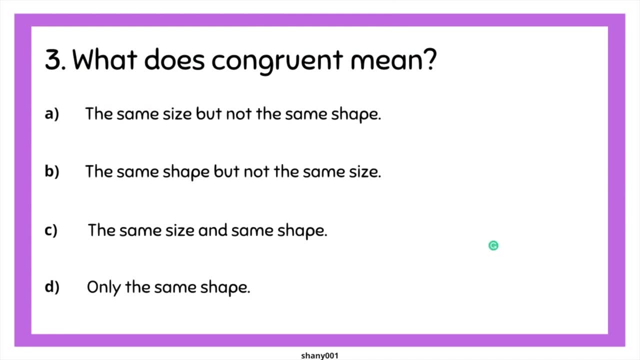 Number three: What does congruent mean? A- The same size, but not the same shape, B- The same shape, but not the same size, C- The same size and same shape, Or D- Only the same shape? Number four: 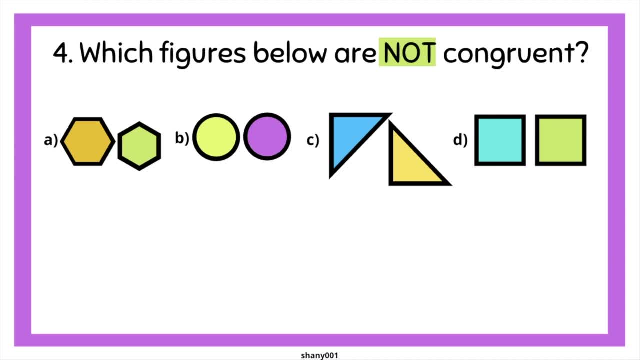 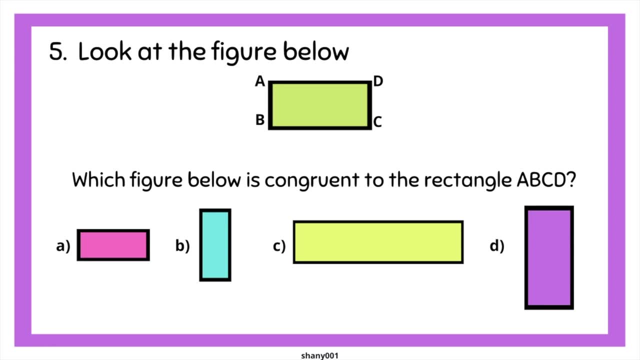 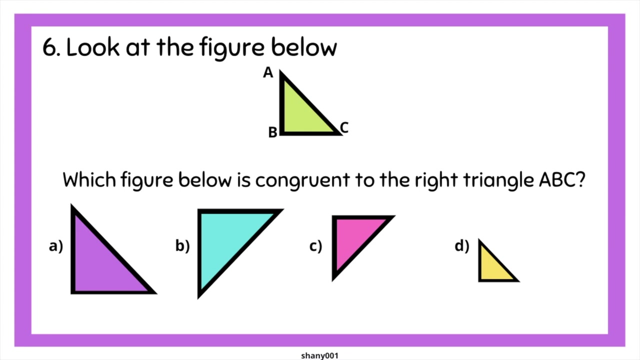 Which figures below are not congruent. Number five: Look at the figure below. Which figure below is congruent to the rectangle ABCD? Number six: Look at the figure below. Which figure below is congruent to the rectangle ABCD? Which figure below is congruent to the right triangle ABCD? 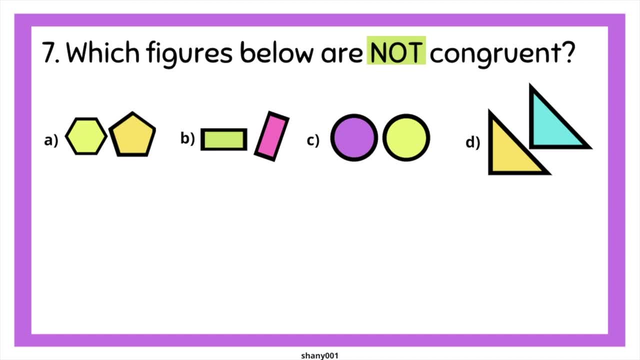 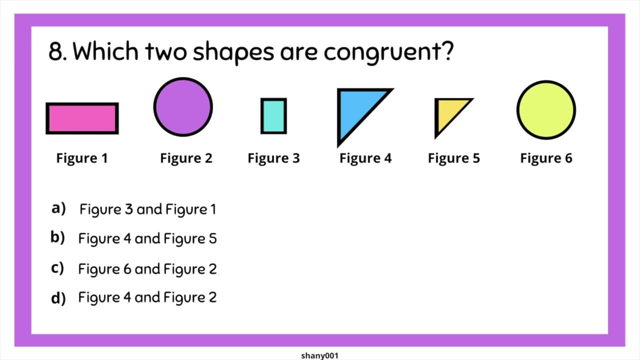 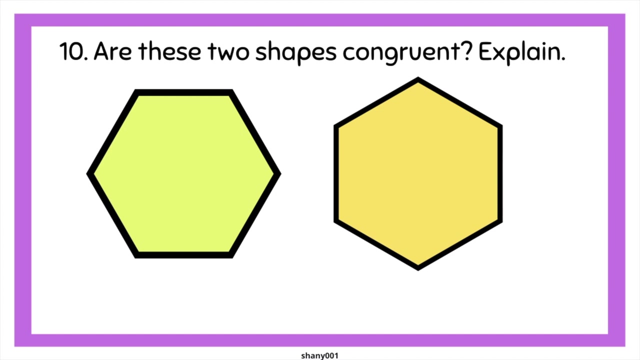 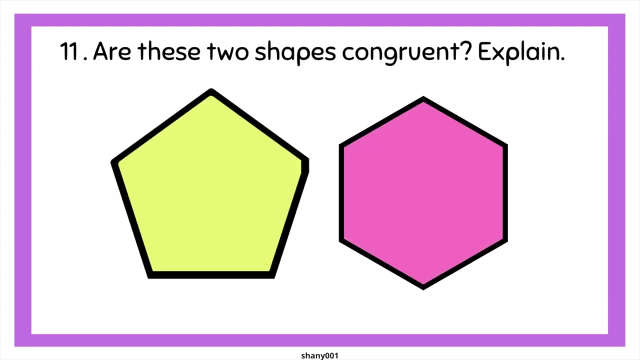 Number seven, Which figures below are not congruent. Number eight, Which two shapes are congruent? Which shapes make up the triangle in the left triangle? Number nine, Which two shapes are not congruent. Number ten, Which two shapes are not congruent. 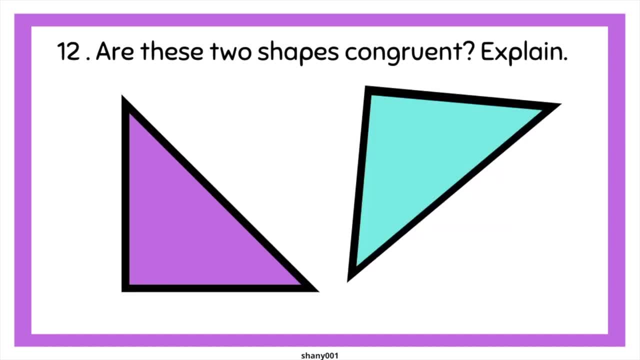 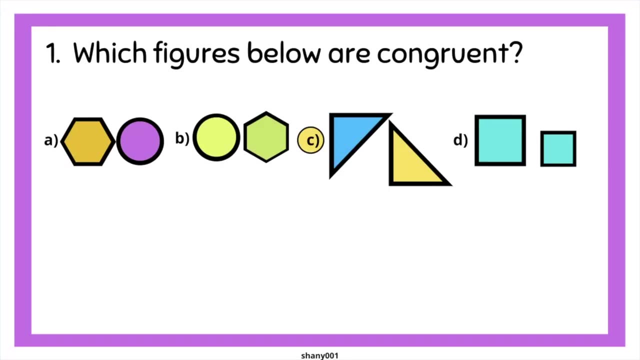 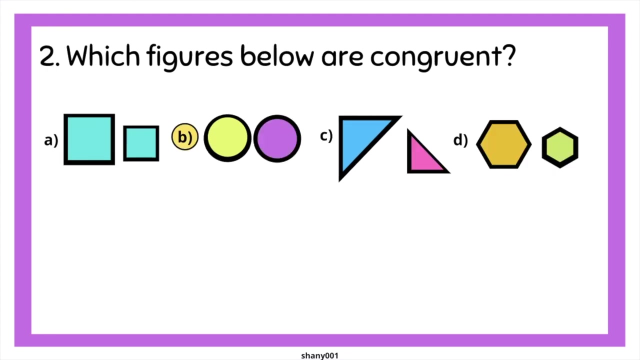 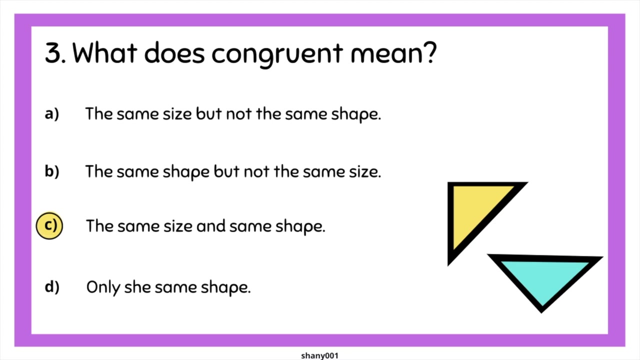 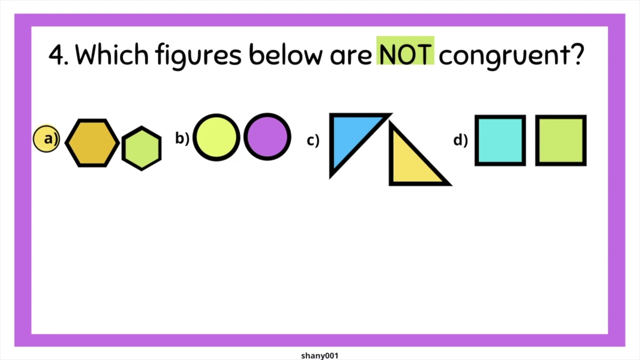 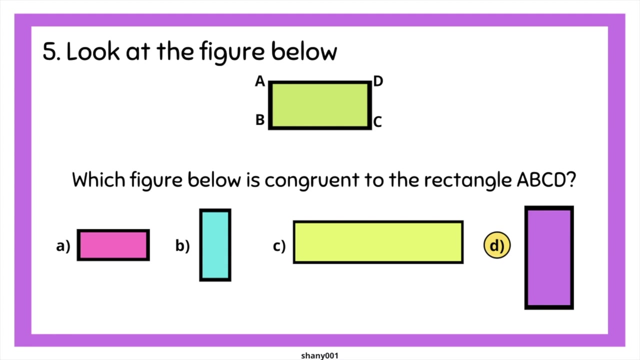 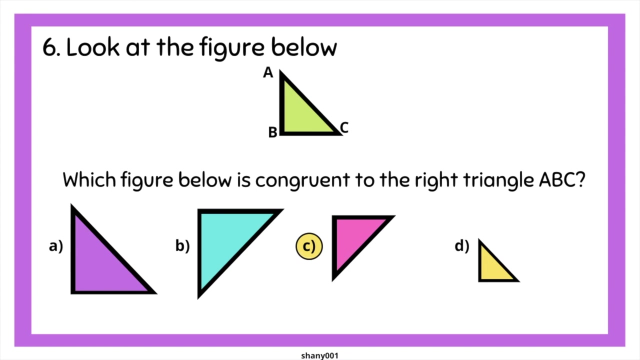 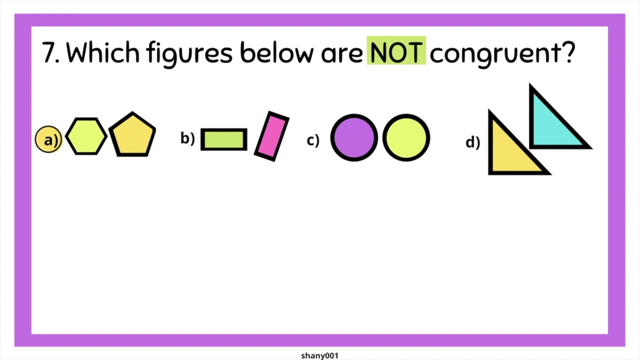 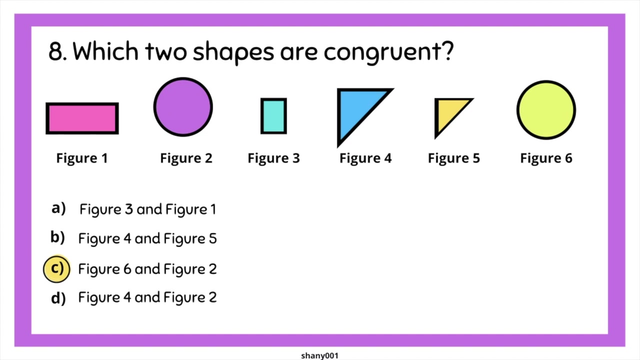 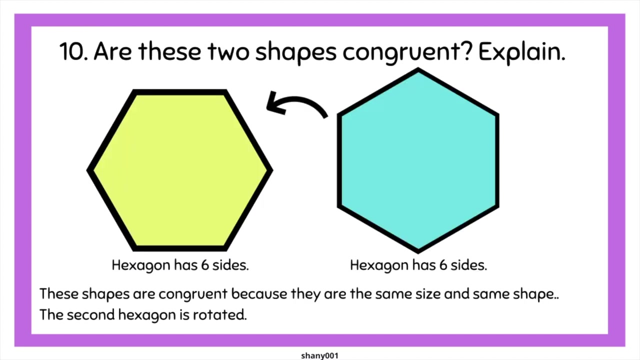 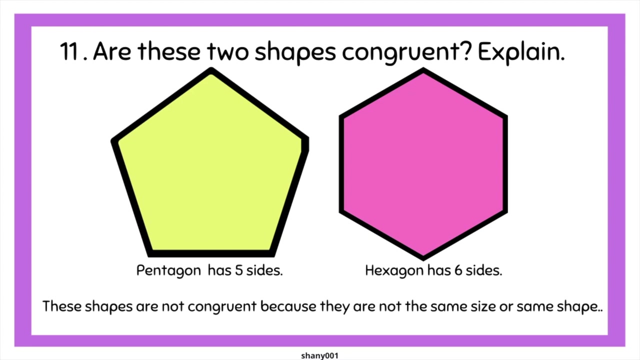 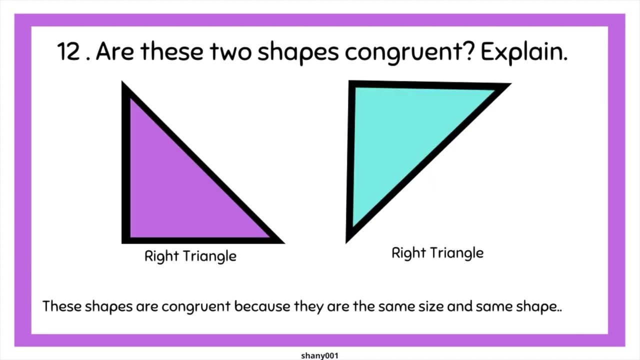